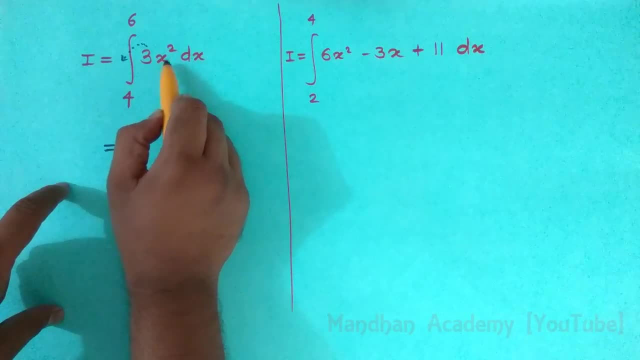 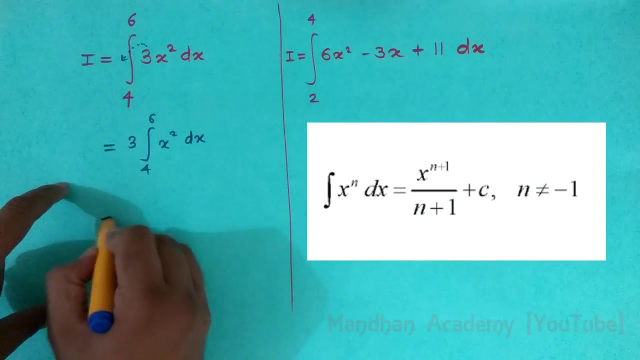 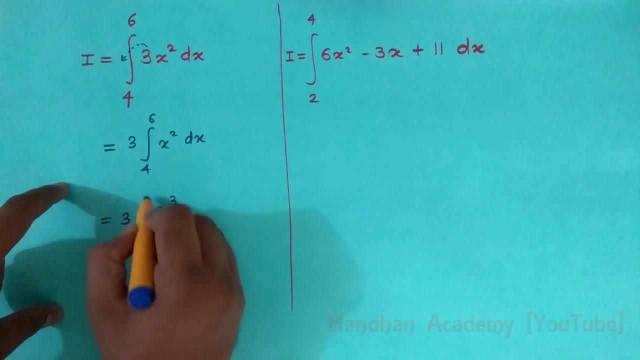 if a number or a constant is getting multiplied with a variable, you can take it outside. So here 3,. these are also called as limits: x, square, dx. Now what is power? rule of integration? This is x raised to n plus 1 upon n plus 1.. Now what you have to do is just put square. 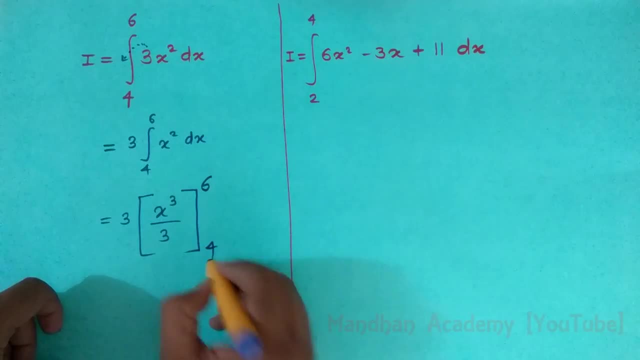 bracket and write down the limits. So you need to remember one thing: upper limit minus lower limit. So in the same function you have to apply upper limit for x. For the same function, you have to apply a lower limit and have to subtract. 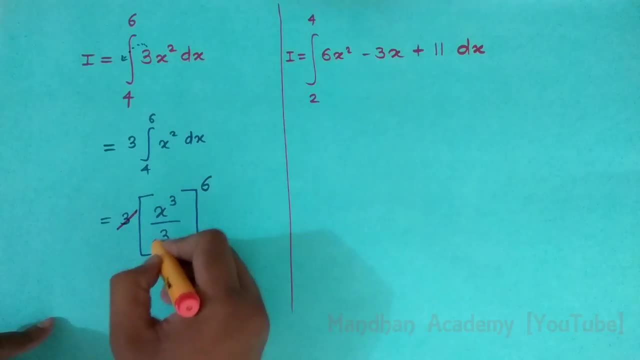 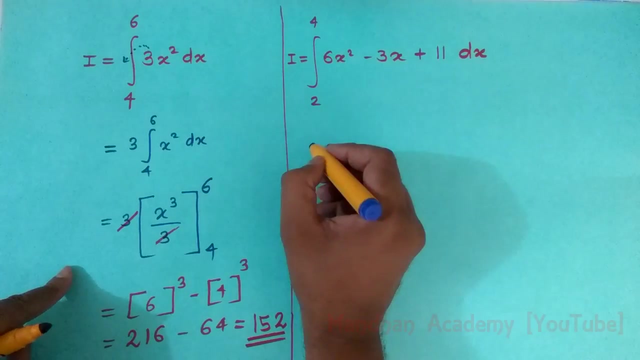 Here you can see that 3 and 3 is getting cancelled. Okay, Now apply upper limit minus lower limit. In every place of x apply upper limit, that is, 6 cube Minus 4 cube. Let's have a look at another example In this question. just you have to integrate the function. 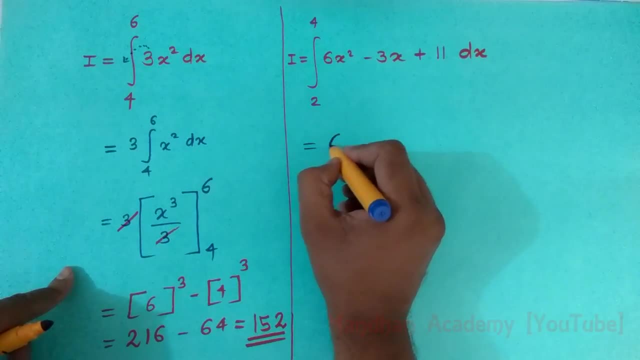 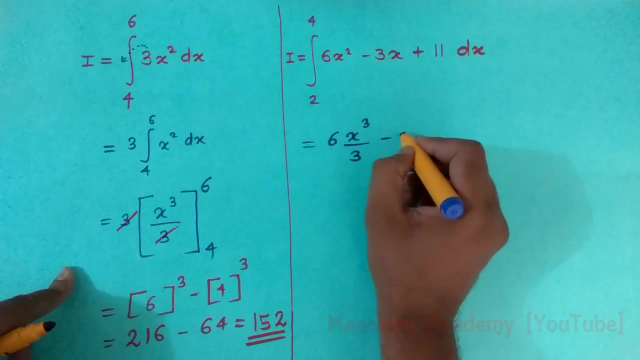 I am going to integrate it directly. 6 outside x square integration would be x raised to 2 plus 1 upon 2 plus 1, according to formula 3 outside Integration of x. Can I say x is x raised to 1?? So it would become x raised to 2 by 2.. 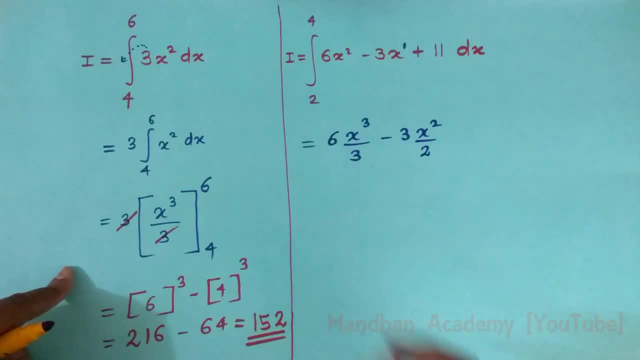 What about integration of 11?? There is one rule of integration: Integration of 1 is x. If integration of 1 is x, according to this formula, integration of 11 is 11 x. So here my answer is 11 x. 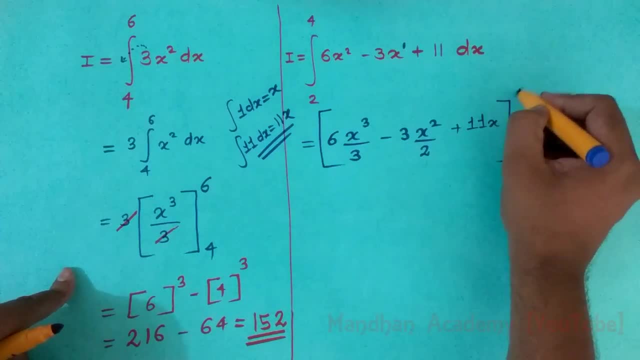 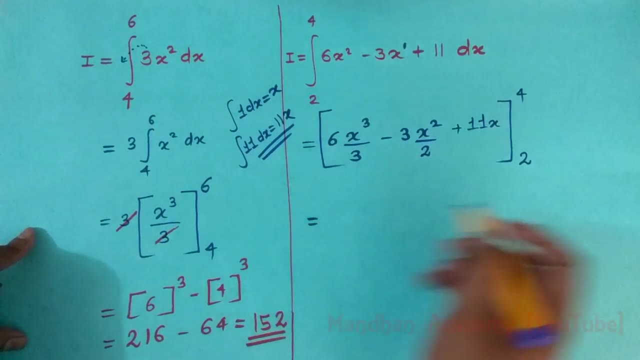 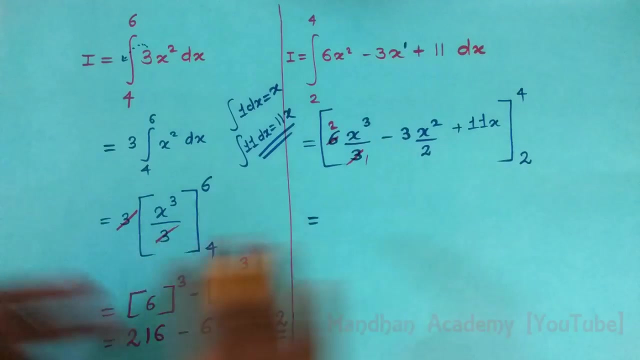 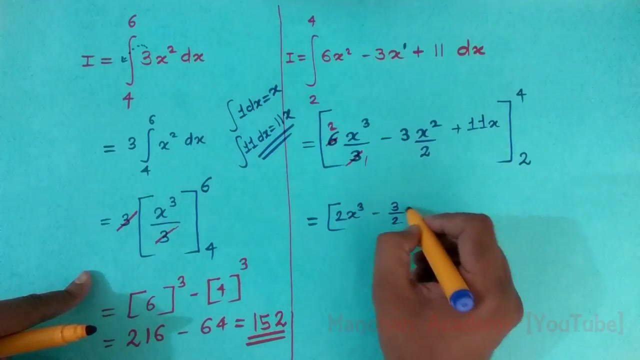 Integration is nothing, just application of formulas. you have to apply the limit and you will get the answer here. something is getting cancelled: 3 1 time, 3, 2 times and nothing else. rewrite the function 2x cube minus 3 by 2 x square plus 11x and the range. 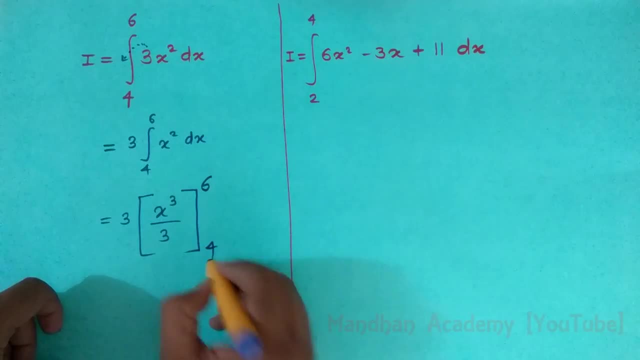 bracket and write down the limits. So you need to remember one thing: upper limit minus lower limit. So in the same function you have to apply upper limit for x. For the same function, you have to apply a lower limit and have to subtract. 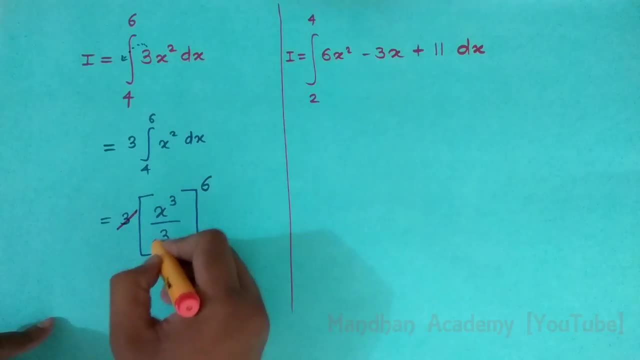 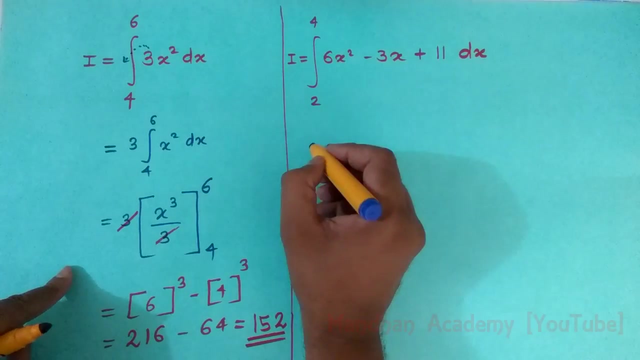 Here you can see that 3 and 3 is getting cancelled. Okay, Now apply upper limit minus lower limit. In every place of x apply upper limit, that is, 6 cube Minus 4 cube. Let's have a look at another example In this question. just you have to integrate the function. 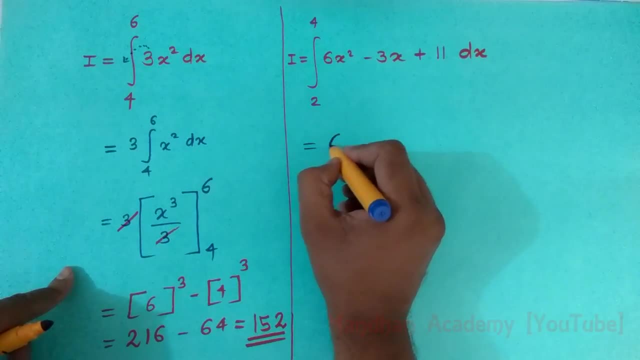 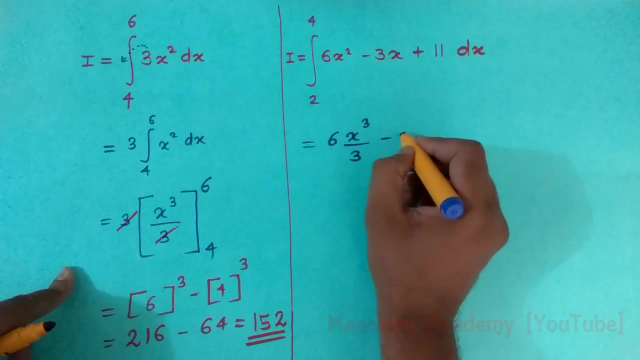 I am going to integrate it directly. 6 outside x square integration would be x raised to 2 plus 1 upon 2 plus 1, according to formula 3 outside integration of x. Can I say x is x raised to 1?? So it would become x raised to 2 by 2.. 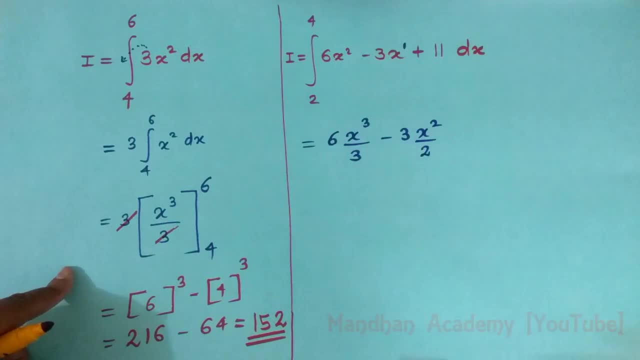 What about integration of 11?? There is one rule of integration: Integration of 1 is x. If integration of 1 is x, according to this formula, integration of 11 is 11x. So here my answer is 11x. 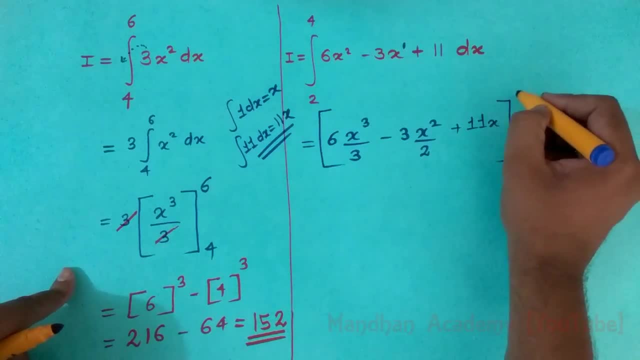 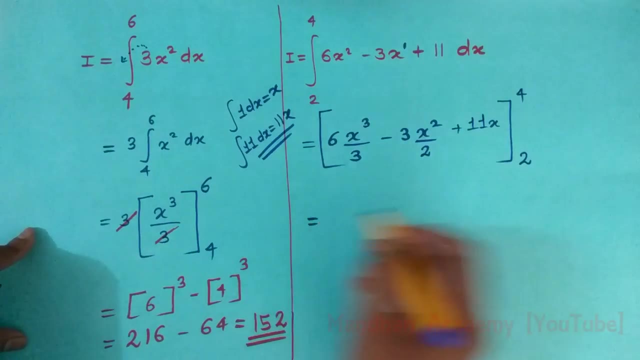 So here my answer is 11x. Integration is nothing, just application of formulas. you have to apply the limit and you will get the answer here. something is getting cancelled: 3, 1 time, 3, 2 times and nothing else. rewrite the function 2x cube minus 3 by 2 x square plus 11x and the range.